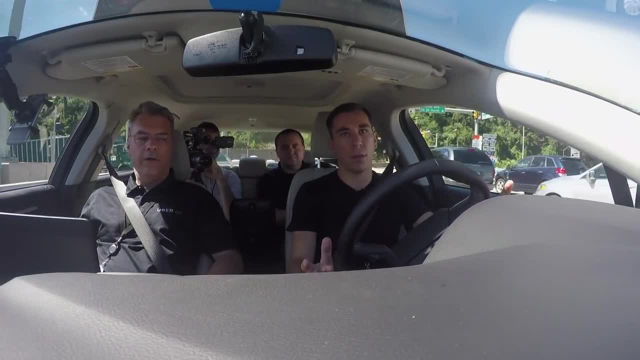 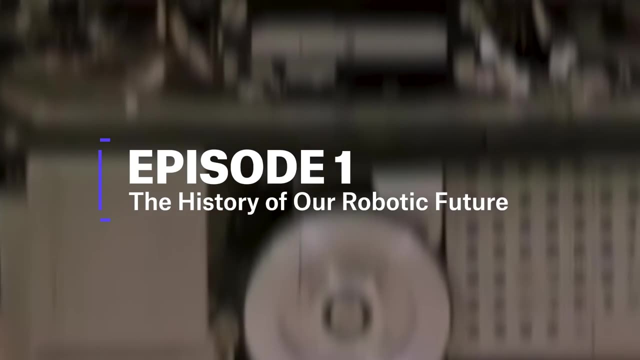 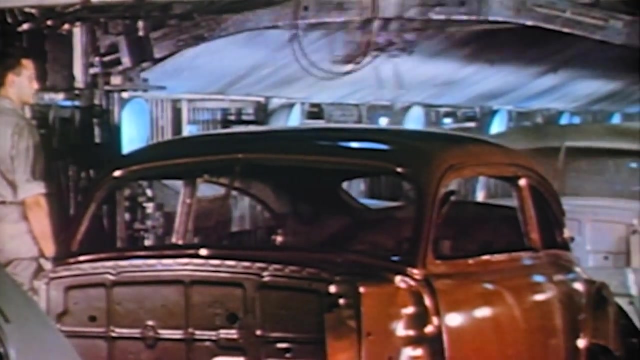 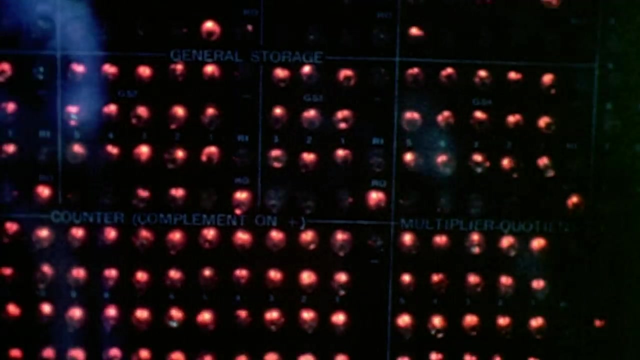 So how did we get here And where are we going? As early as the 1940s, the first modern automation began to show up in factories. Computers were still decades away from becoming personal, But by the late 50s and early 60s computer scientists were already trying to figure out the big question. 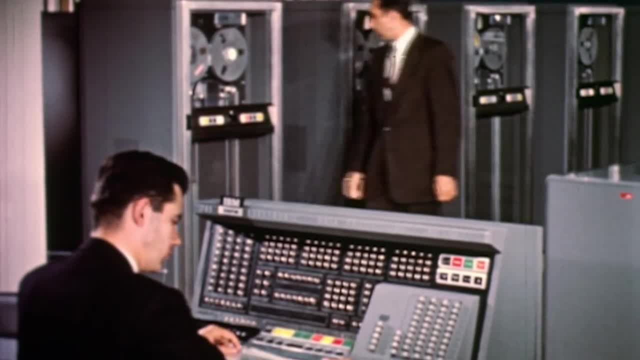 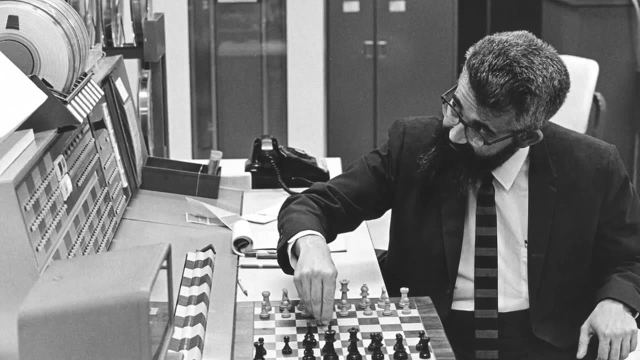 Will robots make our lives better or will they replace us entirely? On one side was John McCarthy with Artificial Intelligence, or AI. You know it was roughly the studying of the internet rules that used AI and AI. that is currently the the beginng. get healthcare ten to make us work at the top. 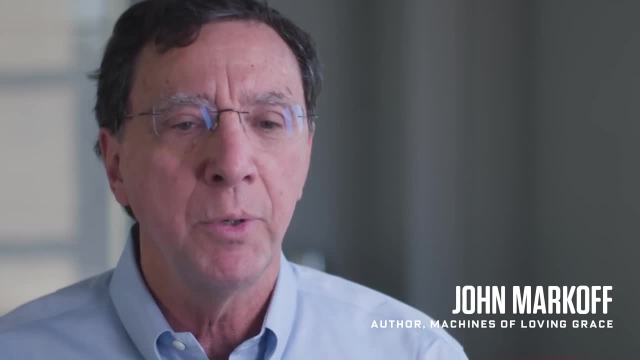 What is difficult for themes like AI- and AI the only few to take a familiar look at- is AI as a model tohen action of a set of technologies that would sort of mimic or replicate human capabilities, whether they were intellectual or physical. 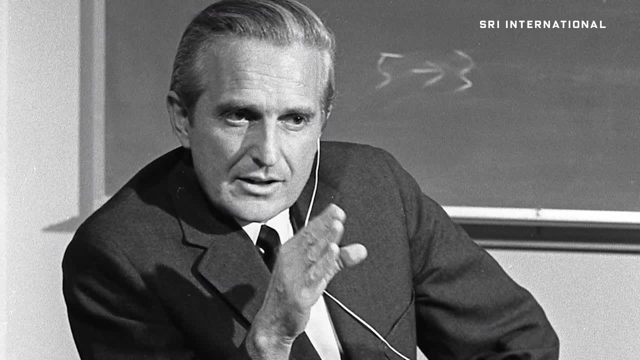 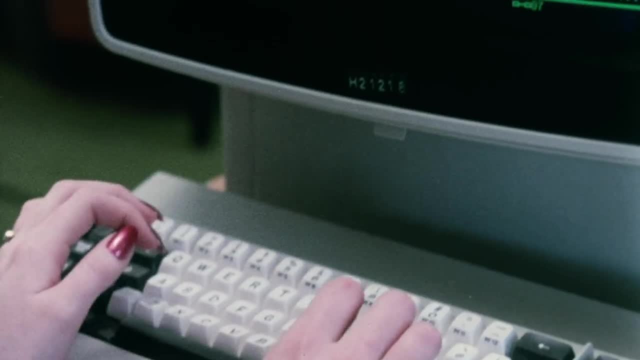 On the other side was Doug Engelbart's idea of intelligence augmentation or IA, And that sort of led to the things that would become the internet and personal computing. So you have these two philosophies and it's interesting they sort of form both a dichotomy. 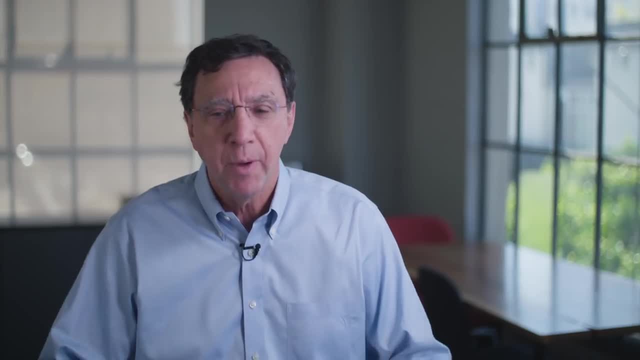 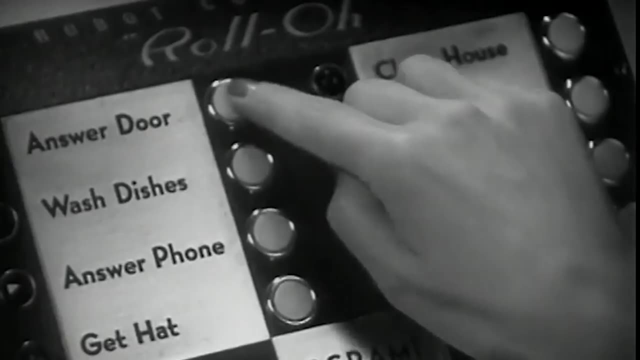 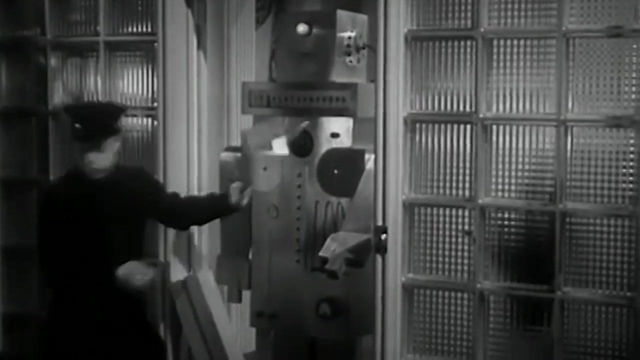 and a paradox: If you extend the human in an IA sense of way- intelligence augmentation- you need fewer machines, Or you can just replace them outright. Robots and thinking machines have long been a science fiction fantasy, But by the 1960s they were actually becoming a reality. 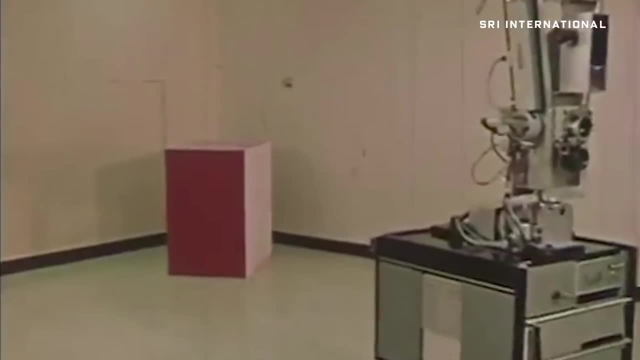 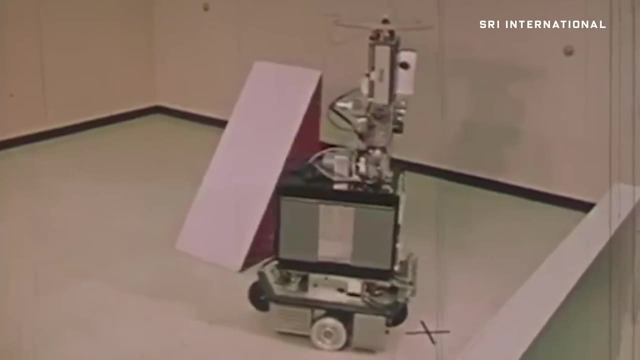 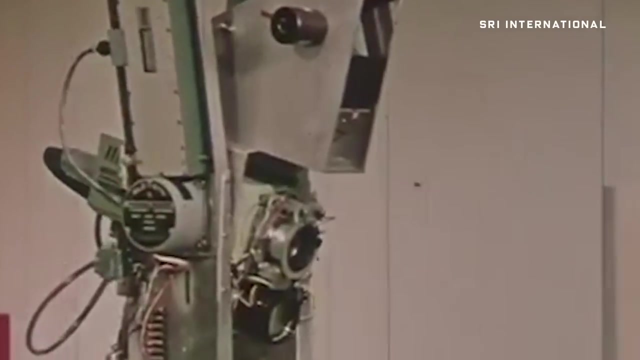 At SRI, we are experimenting with a mobile robot. We call him Shakey, A wobbly, incredibly slow reality. The first real effort to build an autonomous machine that could move and reason and act in its environment was Shakey, Which was: 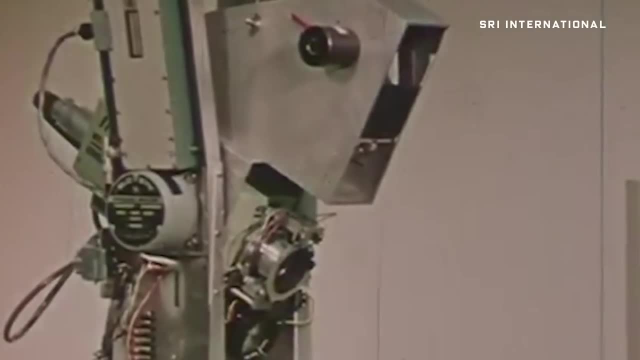 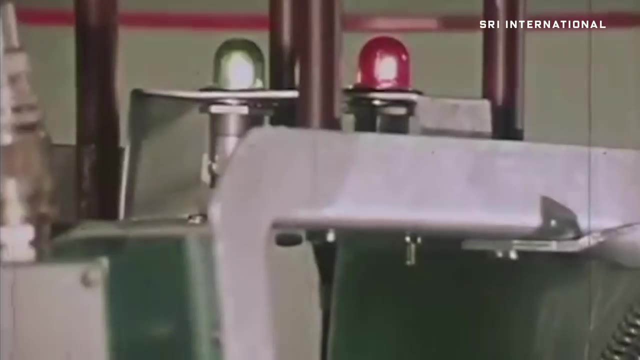 It was a project proposed by a physicist whose name was Charlie Rosen at SRI in 1966. He persuaded the Pentagon by telling them that they could work on a prototype of something that might do reconnaissance or be a guard. At a certain point they asked him how many guns it might carry and he said: well, two. 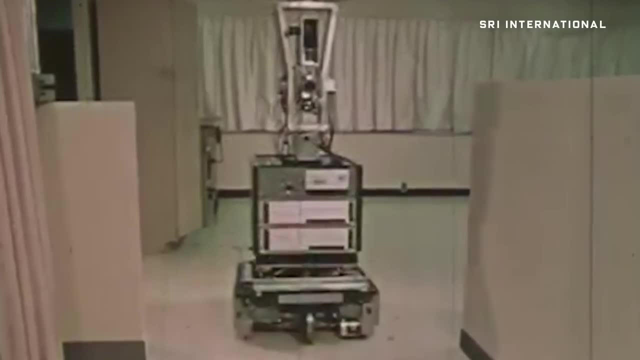 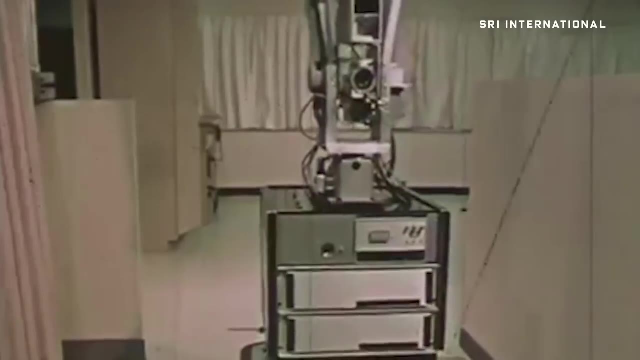 three. how many do you need? While Shakey never carried guns, it did mark the beginning of a new era of computer science. It was important because it was a platform on which the algorithms that would later be used by self-driving cars- The kinds of things that you use in your. 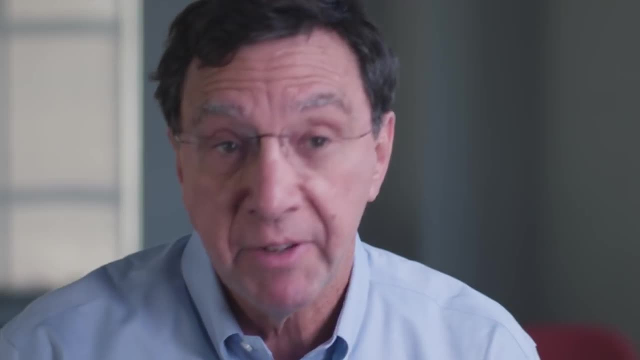 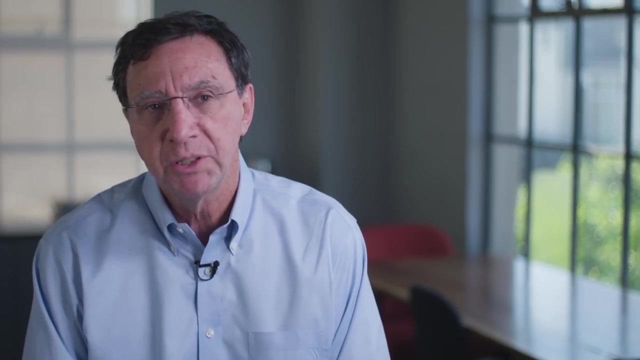 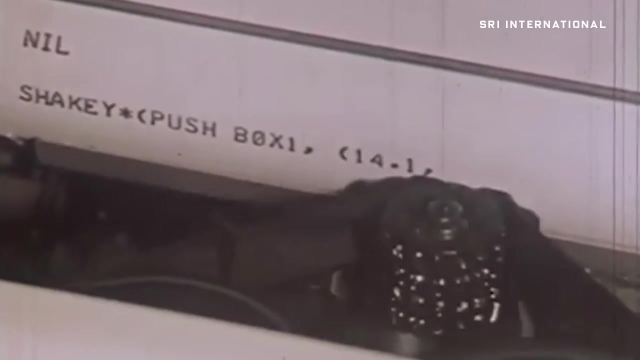 Smartphone, there was an algorithm called ASTAR that was a navigation algorithm, is the sort of granddaddy of the way we get around with our smartphones And I think, importantly too, that the first work on speech recognition that was significant was done in Shakey, because they were looking for some way to interact with the machine. 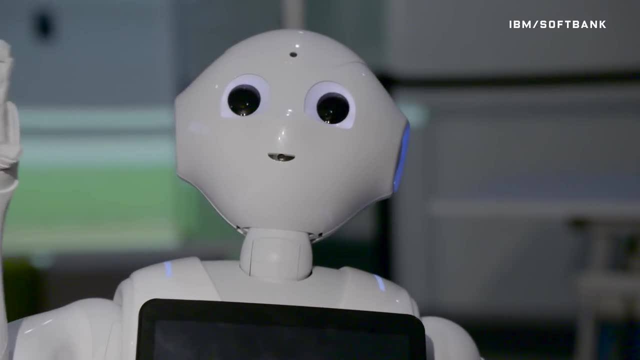 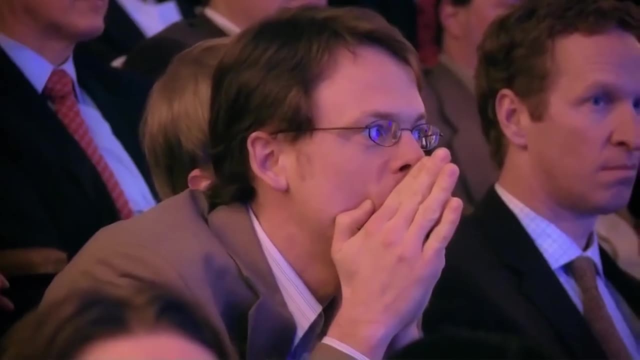 Since the days of Shakey, computers have advanced remarkably in their ability to think for themselves. Advanced AI has beaten humans at their own games, From chess. Now we come to Watson, to Jeopardy. Here's Graham Stoker and the wager. 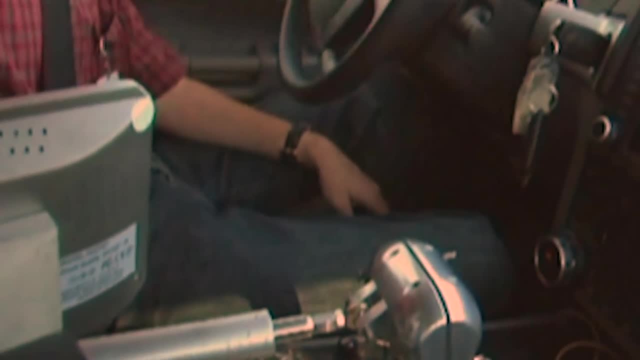 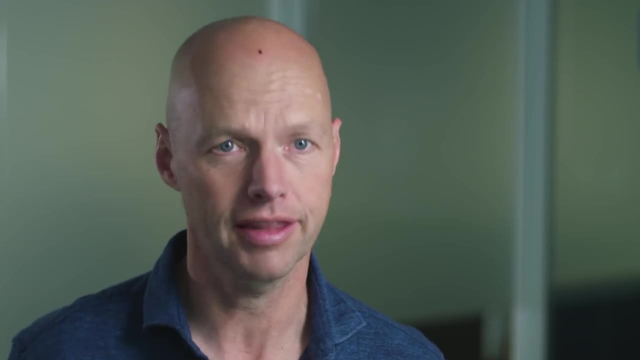 Perhaps most tangibly of all, cars began driving themselves. Twelve years ago. the idea that a computer could drive a car was completely unthinkable. People felt something as intuitive and as hard to even explain as driving a car was reserved for the human race. 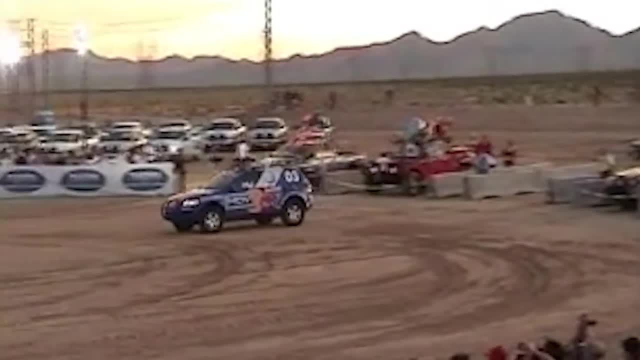 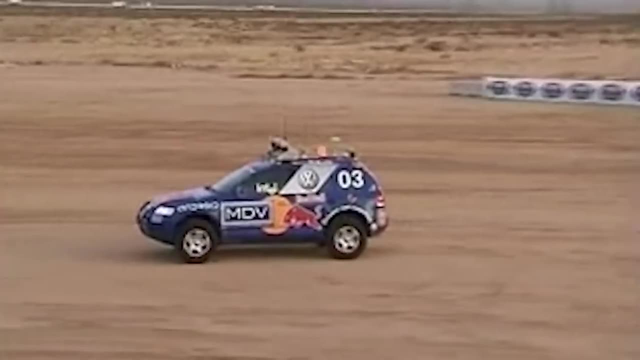 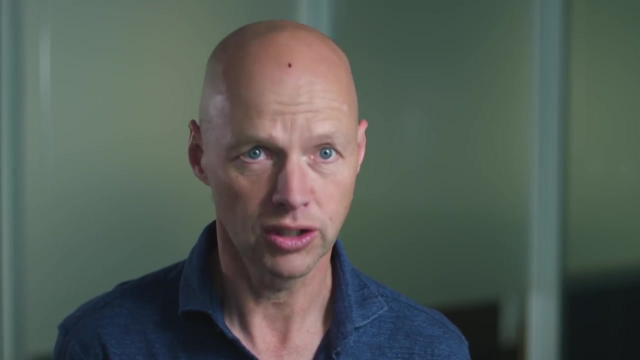 Then the federal defense agency, DARPA, put on a self-driving car challenge. Stanford's team, led by Thrun, won By building Stanley a robot car that drove itself 132 miles across the desert. Our secret ingredient was AI. It was machine learning. 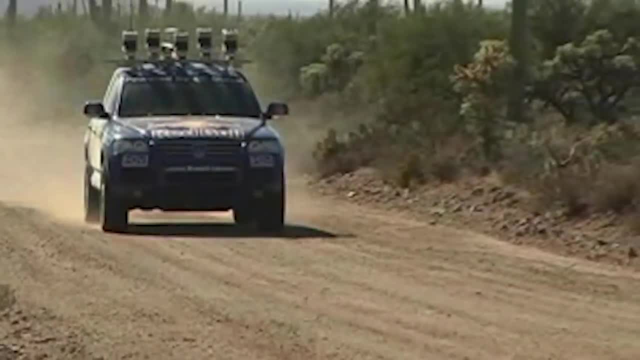 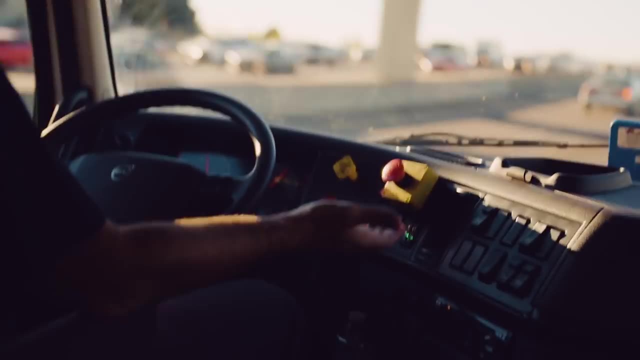